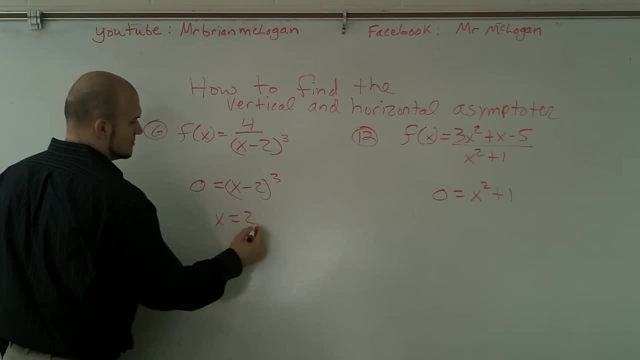 go ahead and do this. I go and factor this: I get x equals two. okay, I don't have to do that. take a cubed root on both sides. you guys need to show that you okay with that. take a cubed root. I'll just show it: cubed root on both sides to get rid of the. 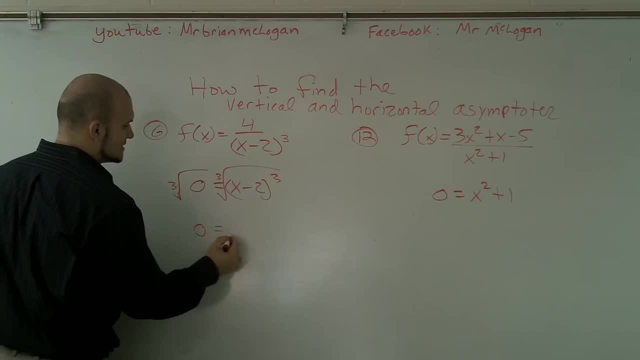 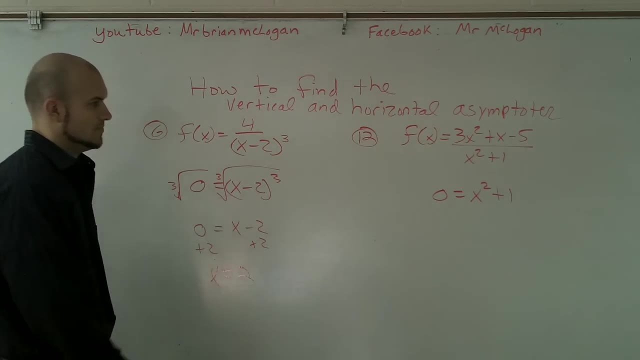 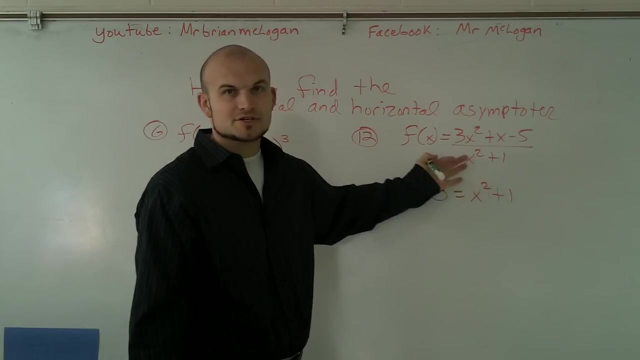 cubed. okay, therefore, then you have: zero is equal to x minus two. add a two on both sides: x is equal to two. okay, Over here I notice that there is no number. that is, that's going to be an imaginary number, right? 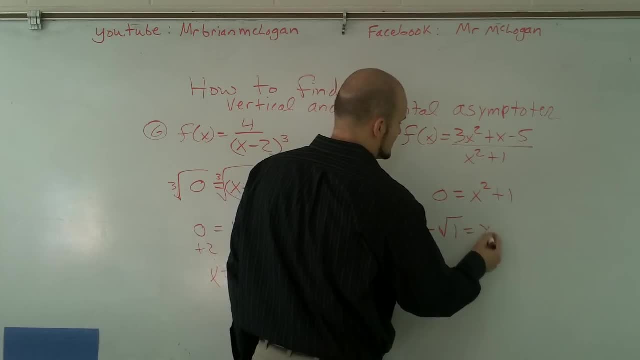 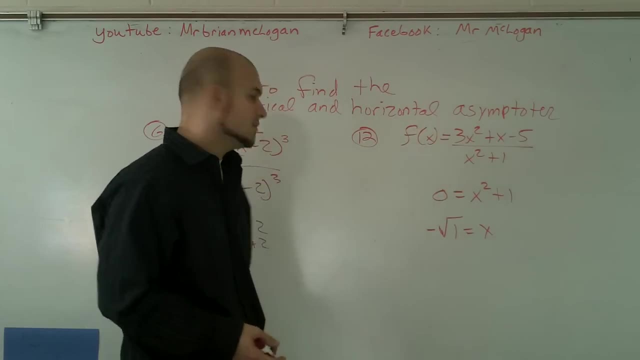 That's going to be. i squared root over on equals x. right, we worked on taking the i because that's going to be negative. you take the order, it's going to be square root of negative one. So therefore, there is no x. there's no x intercepts or vertical acetopes. 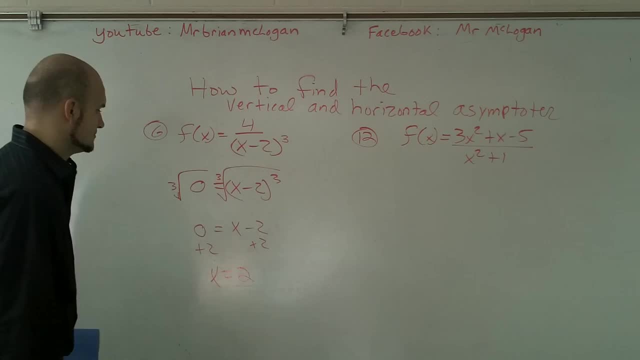 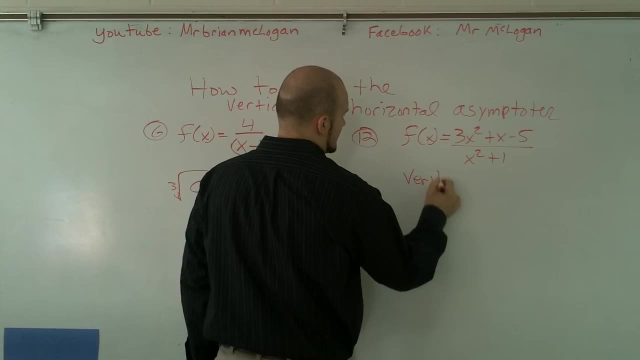 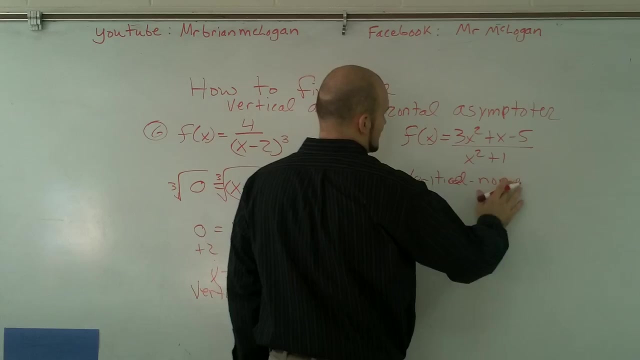 over here. Then for the horizontal, so that's your vertical, and for here vertical, we have none. I don't know why I did the double v. And now to go ahead and find the horizontal acetope. remember the horizontal acetope. 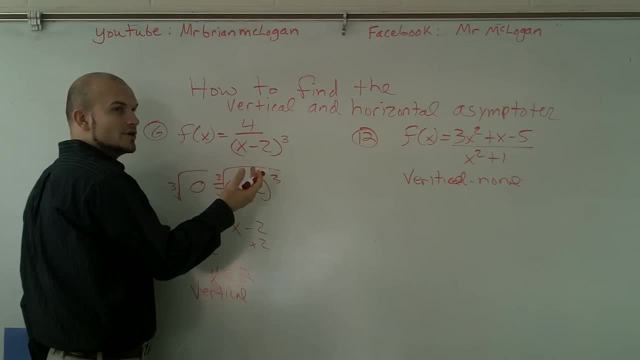 what we need to do is we need to look at your exponents of your leading coefficient and if we have our leading, if our degrees up, here is what we look at and here you can pretty much write: we have x to the zero right, because there's nothing written there. 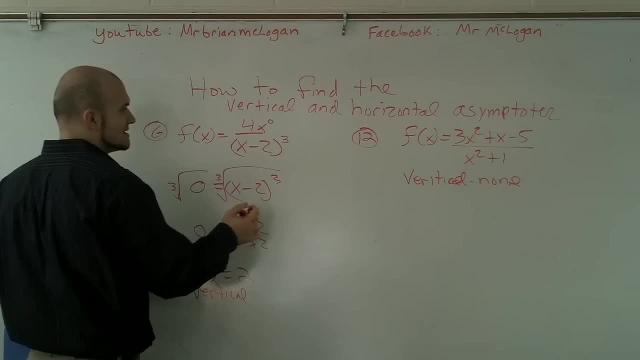 so it's x to zero. So, if you guys remember what we wrote down, last class period is when you go ahead and compare This. eventually, if I in fact FOIL this all out, I'm going to get x cubed right. 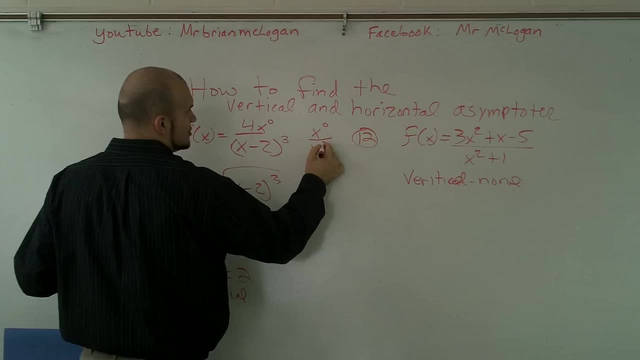 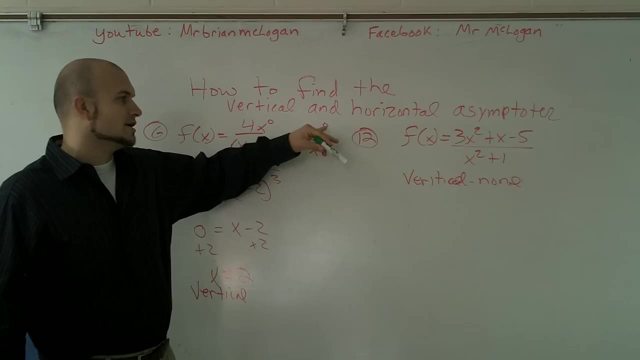 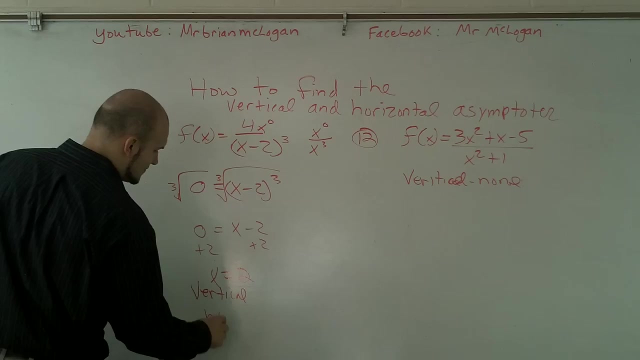 So essentially what I have is my $2 x over x cubed, and if you guys remember that, whenever your the degree in the numerator was less than a degree in the denominator, therefore you had a horizontal acetope of zero. So therefore you're right. 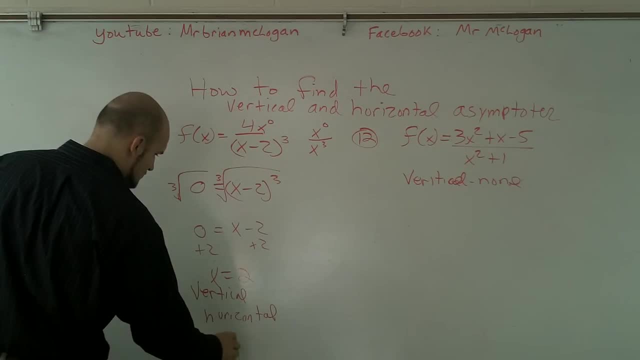 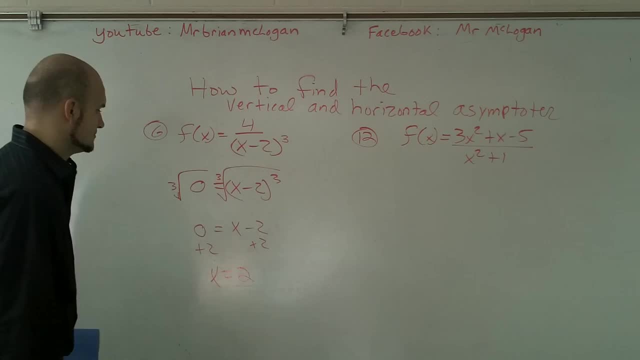 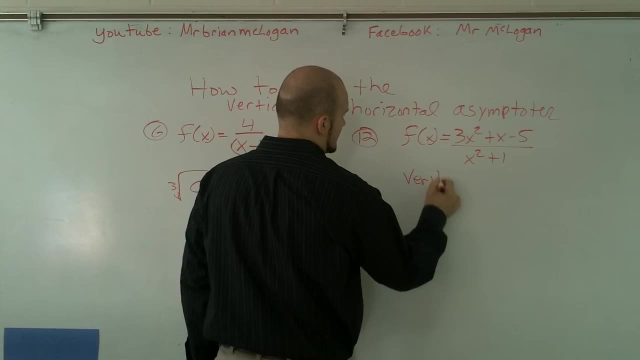 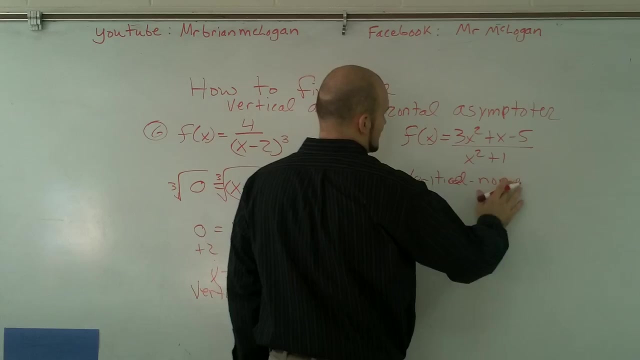 over here. Then for the horizontal, so that's your vertical, and for here vertical, we have none. I don't know why I did the double v. And now to go ahead and find the horizontal acetope. remember the horizontal acetope. 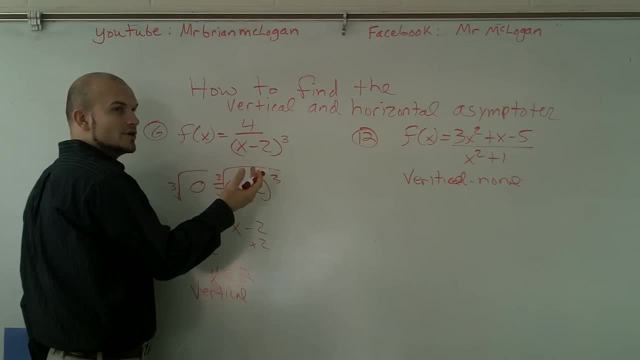 what we need to do is we need to look at your exponents of your leading coefficient and if we have our leading, if our degrees up, here is what we look at and here you can pretty much write: we have x to the zero right, because there's nothing written there. 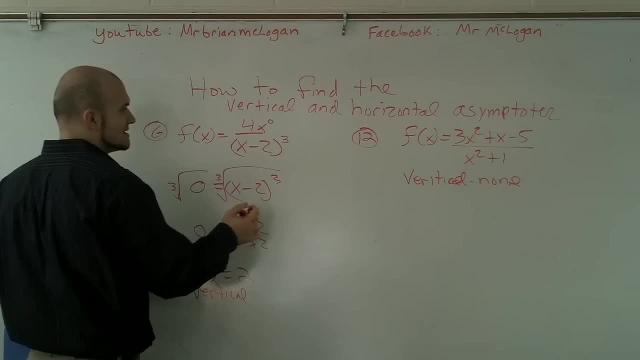 so it's x to zero. So if you guys remember what we wrote down, last class period is when you go ahead and compare. So this: eventually, if I back, FOIL this all out, I'm going to get x cubed right. 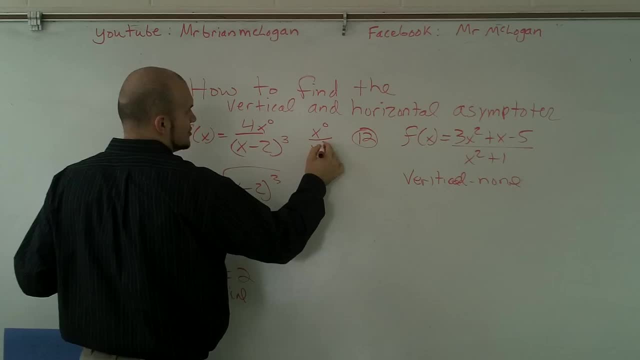 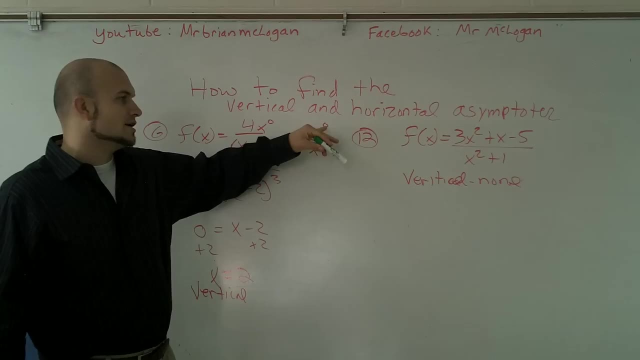 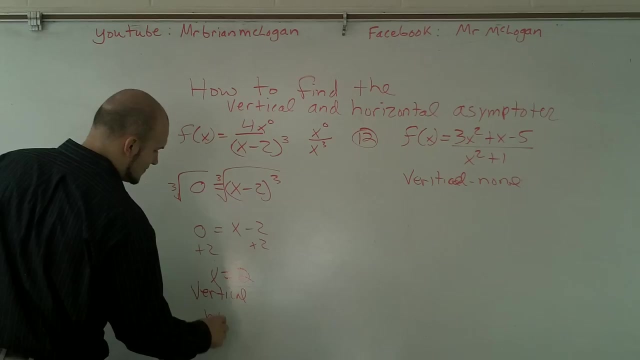 So essentially what I have is my $2, x over x cubed, And if you guys remember that whenever your denom, the degree in the numerator was less than the degree in the denominator, therefore you have a horizontal acetope of zero. 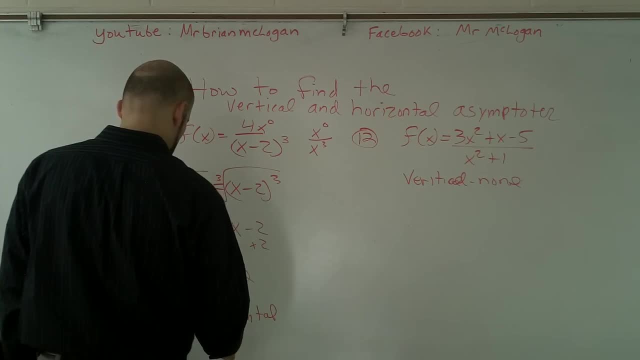 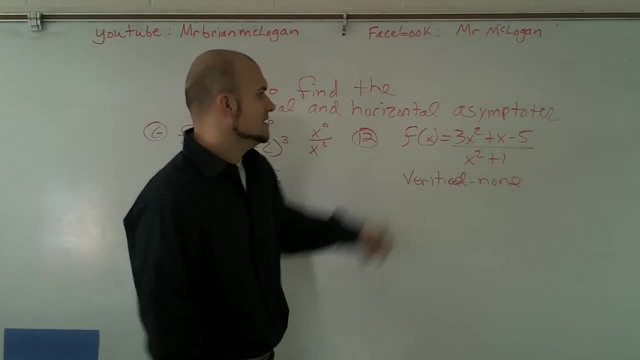 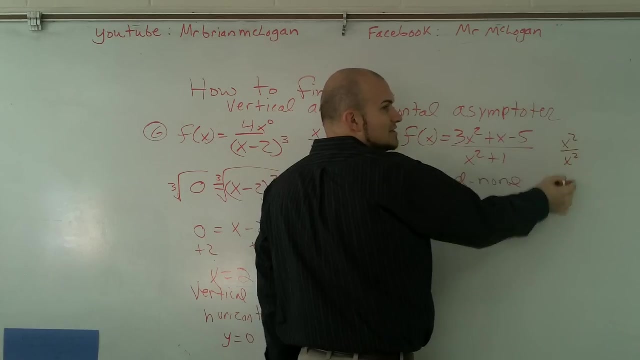 So therefore your four, Okay, Okay. So the vertical is this: horizontal equals y, equals zero. All right, And then for number 12, now we notice that we have: x squared is equal to x squared, right, So we have. when I'm looking at my leading coefficients, now these are equal to each. 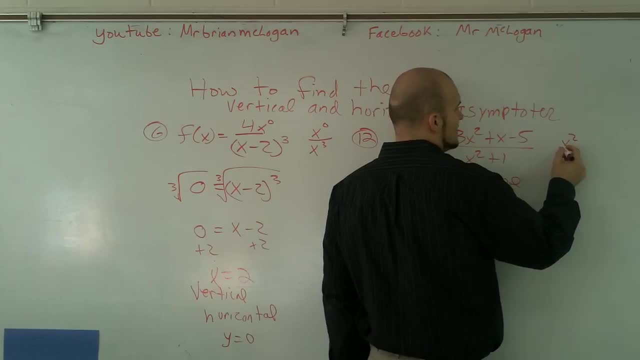 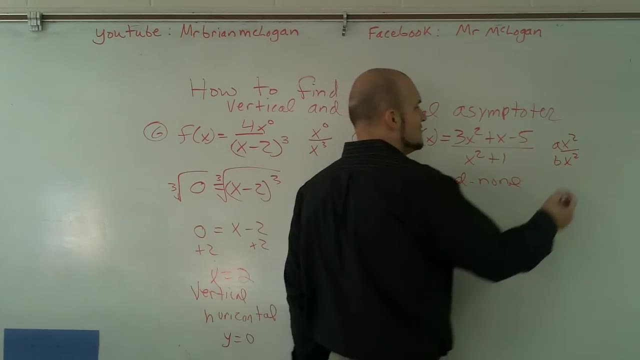 other. So when they're equal to each other, we have A and B is what we call their coefficients of them, And what they do is when you have, when you have, 2 is equal to 2, you, when you have their. 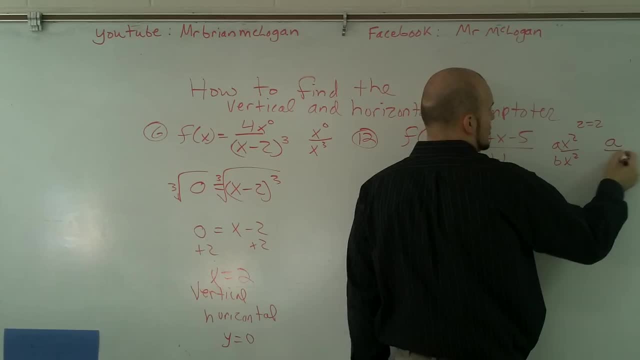 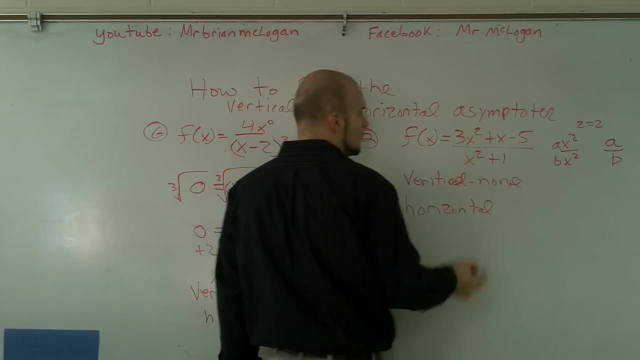 degrees are equal to each other, then the horizontal acetope is the ratio of A over B. So the horizontal for this problem is going to be 3 over 1, because the coefficient for this problem is 1. So it'd be 3 over 1.. 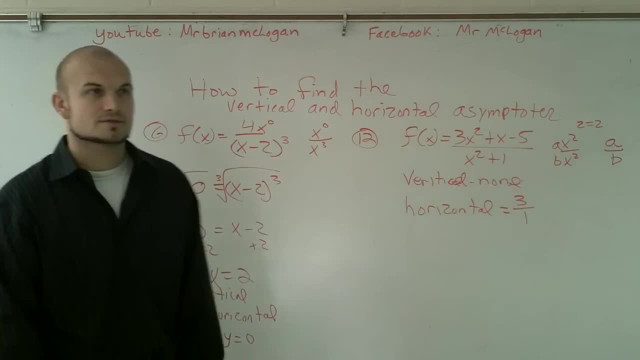 So that's how you find the vertical and horizontal acetopes of given functions. What was the domain? Okay,